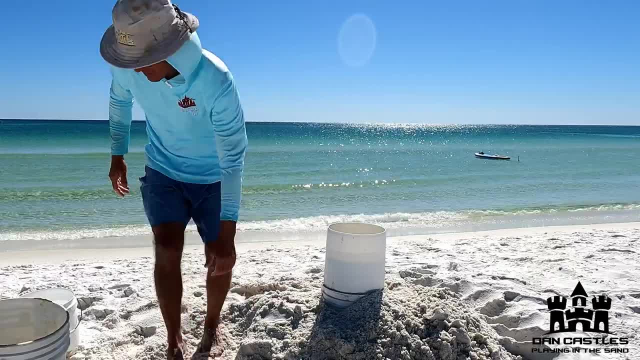 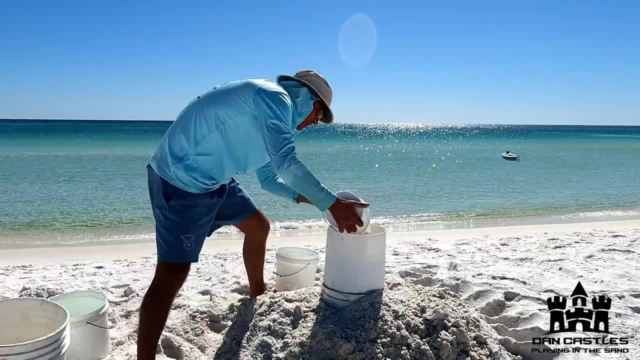 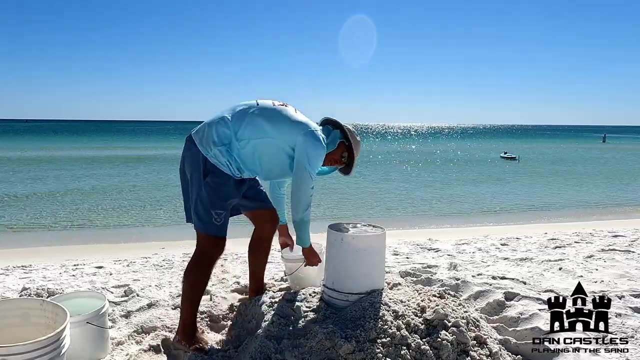 Any garbage, Grab it and throw it out. We're done with those layers. We still have water in here. That's good. That's an A plus in sandcastles. We're going to add more dry sand to that layer. Bring about an inch from the top. Just enough room to get some water in there. Water, water, water, water, water. You can never use too much water when building a sandcastle this way. 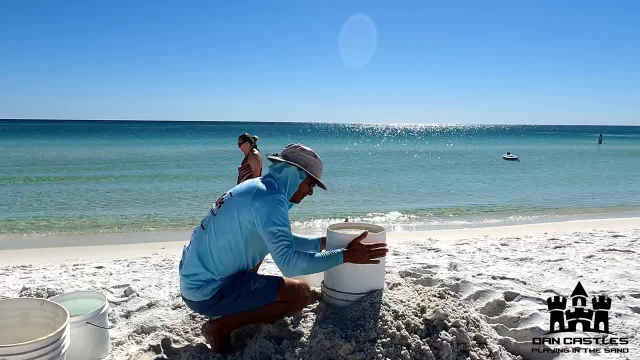 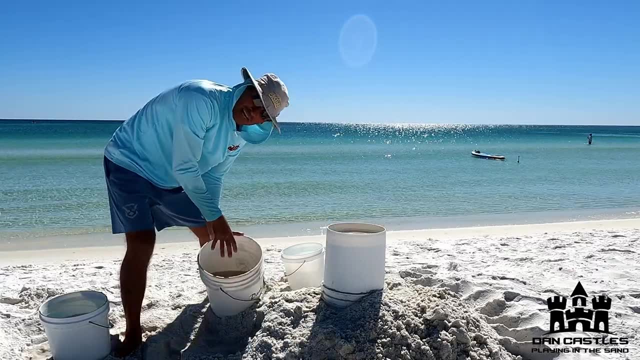 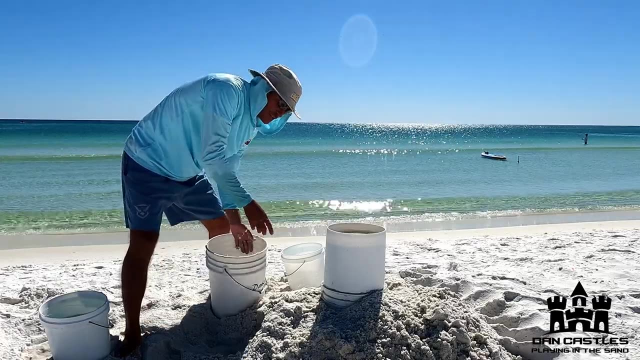 It's mixed Tap, It's all tapped. You're really close to the top. You don't want to continue with dry sand. Take a bucket, Put more sand or more water than sand in it, So down at the bottom here I got this really soupy, watery sand. I'm going to use this to finish it off. 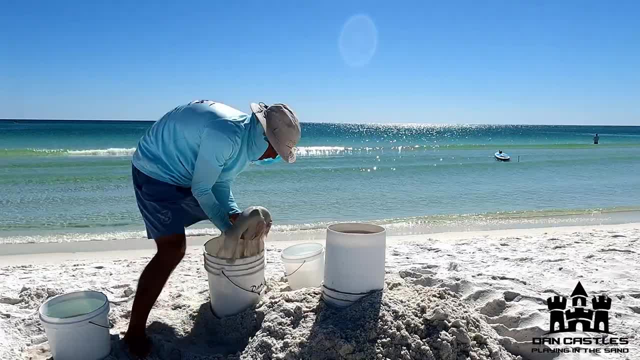 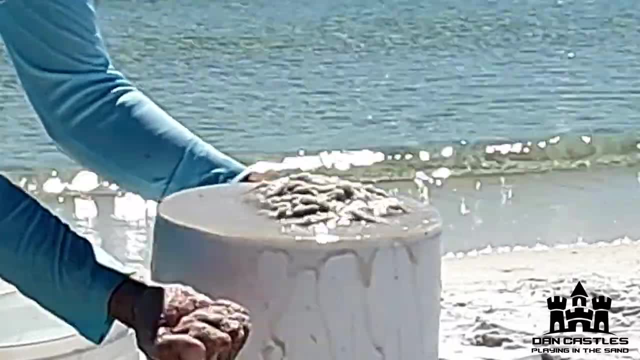 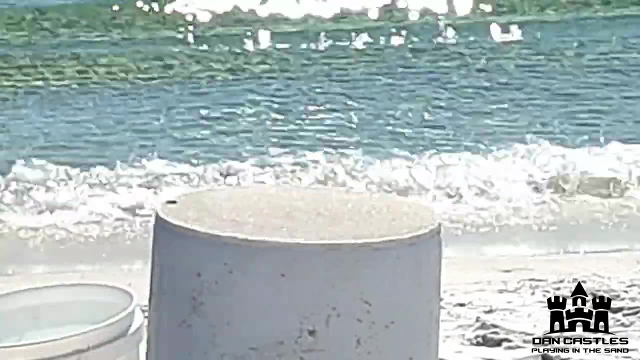 While there's still water, big handfuls of sand, Big handfuls of sand All the way to the top Fist bump. Vibrations cause it to settle off smooth. Whizz it, All right. Whizz it Ta-da. 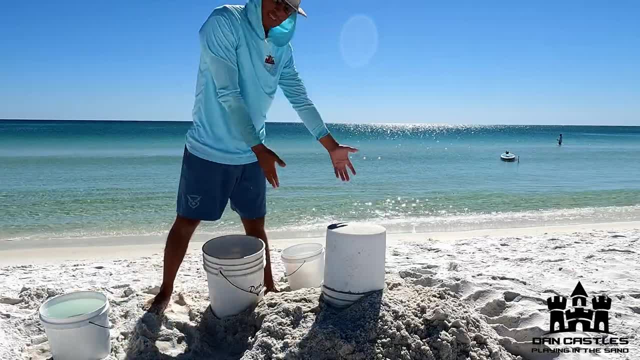 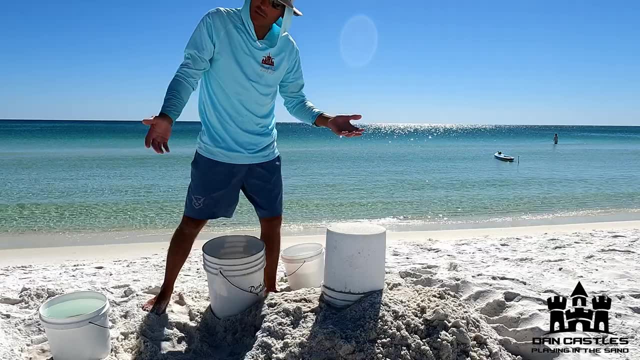 And that is how you successfully build a sandcastle in Destin, Florida. Like I said, this doesn't work everywhere, so experiment on your beach. Some beaches require more water. Some beaches require less water. Some beaches- this isn't going to work at all. 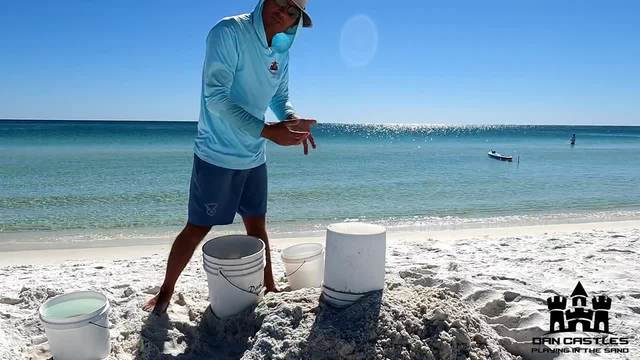 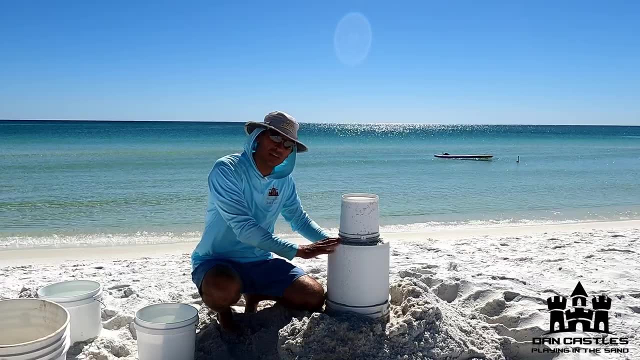 You can even do this on a riverside beach. You just have to figure out the right formula. but I promise, if you follow these steps, it will work for you. Okay, now, after your castles, sit here for about a minute or so. you want to let a little bit of that water drain out. 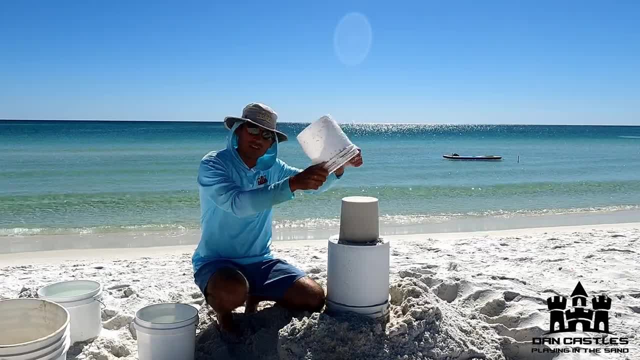 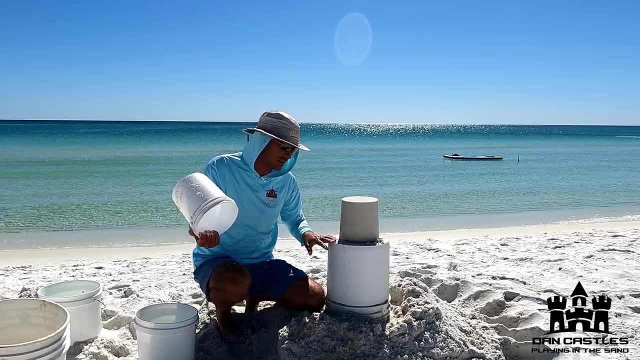 You can come in and you can pop off your forms. They just slide up that easy. The reason why this came out so smooth is because I pre-treat all of my forms before I build a sandcastle. Now, I've been doing this for seven years. 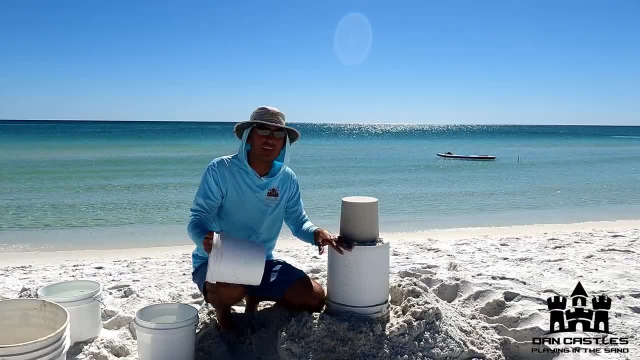 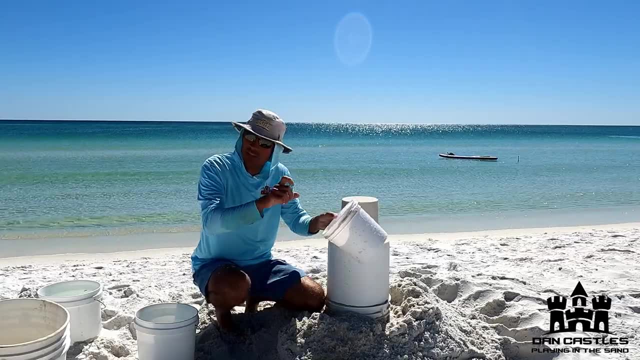 The one thing I found that works the best is WD-40.. WD-40 is hands down the best lubricant I've used to spray on the inside of my buckets. I don't use a lot, Just a little, And that's about it. Two little sprints and you're good to go okay. 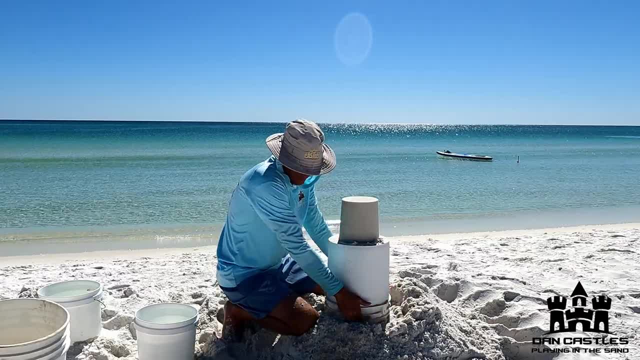 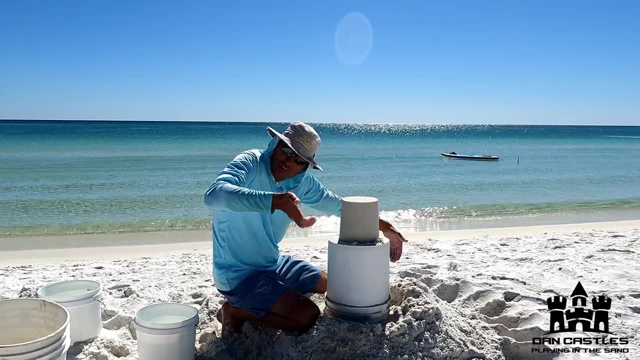 And you can see, just with a little WD-40, once you clean off around the bottom of your buckets and you get your finger underneath and I just curl my fingers up like that, I literally do a finger curl, like, ah, finger curl.